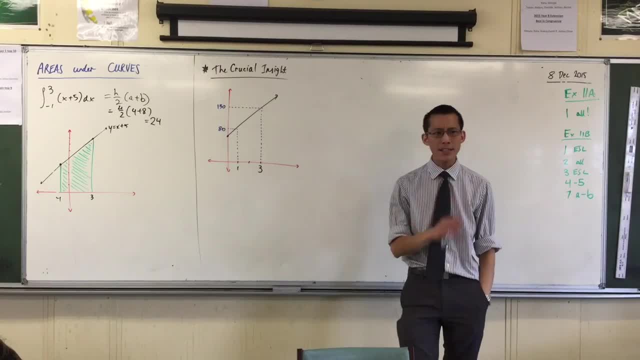 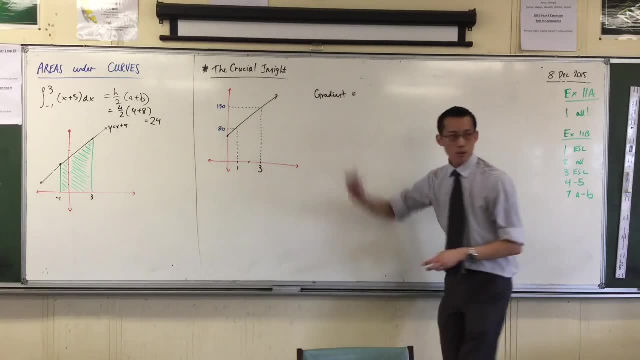 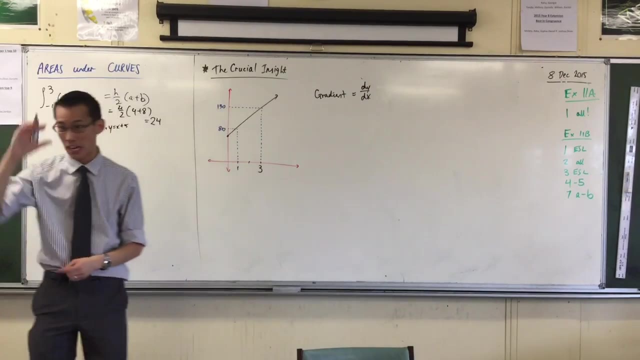 Like, where is it at a given time? The reason why I'm appealing to this is because the idea of gradient, right gradient- being rise over run, which we write in fancy notation as dy on dx: change in y, that's rise. change in x, that's run, okay. 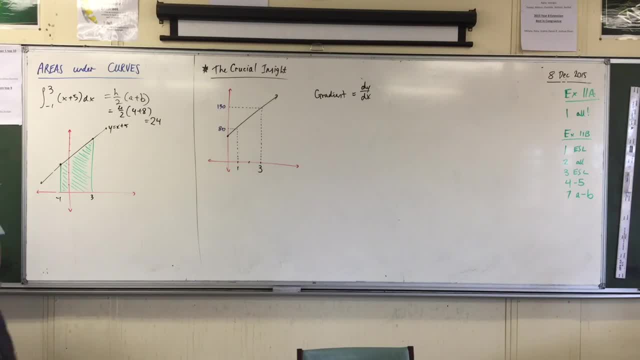 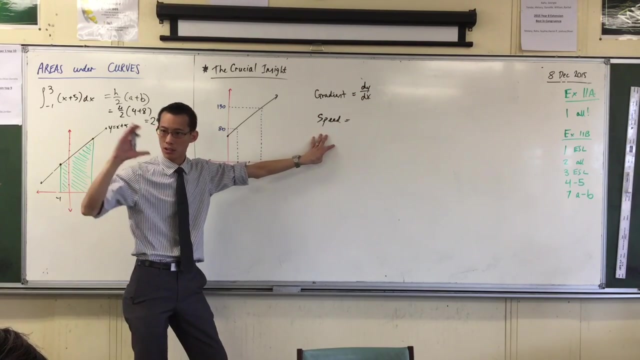 This gradient relationship is exactly analogous to something that a travel graph tells us about, Namely in terms of things moving around. gradient is how something is changing in regard to something else, which is exactly what speed is right. What is speed compared to the changes of two different things? 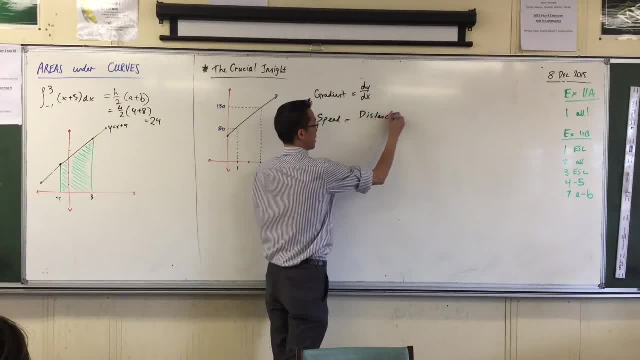 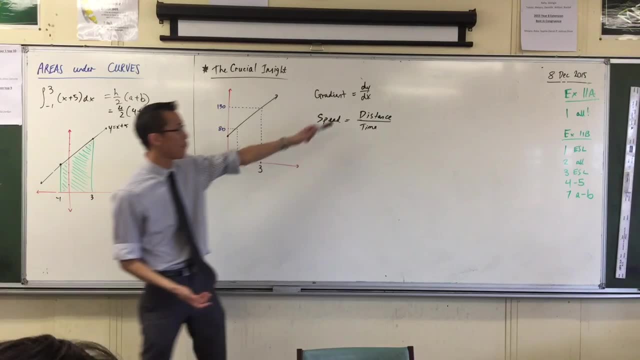 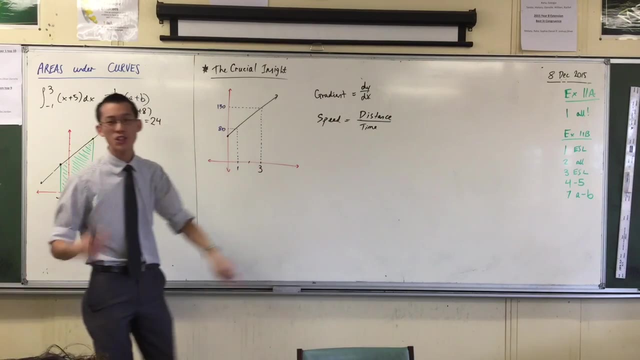 Distance and time. very good, Excuse me. so, for instance, if I travel for five hours and I pass, you know, 80 kilometers in distance, then, I've excuse me, my speed will be 80 over 5, which is 16 kilometers an hour, right? 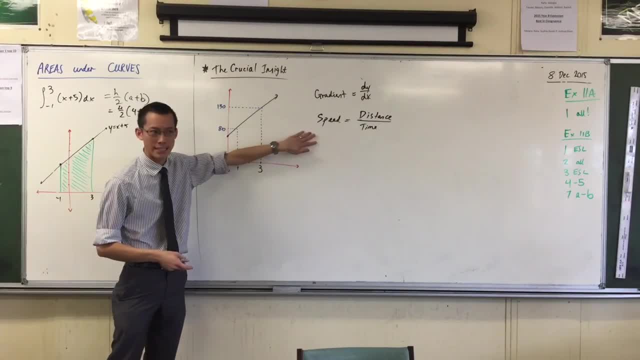 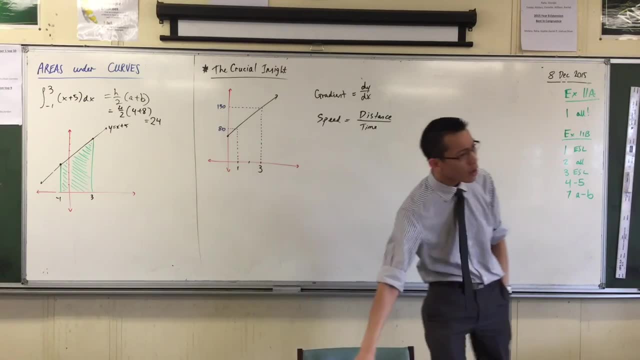 So speed equals distance on time. Now I'm going to take this idea and we're going to try and squeeze some insights out of it. okay, Now have a look at this travel graph with me. What I want you to consider is: we start at a time zero. 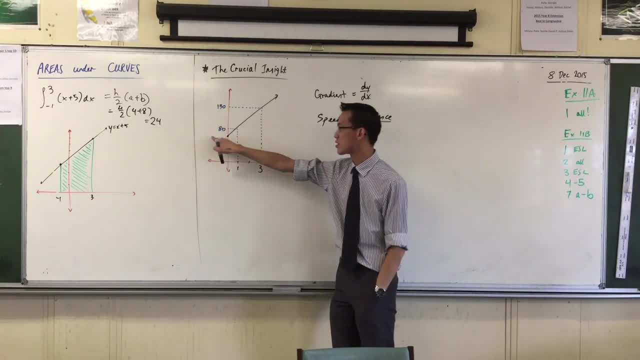 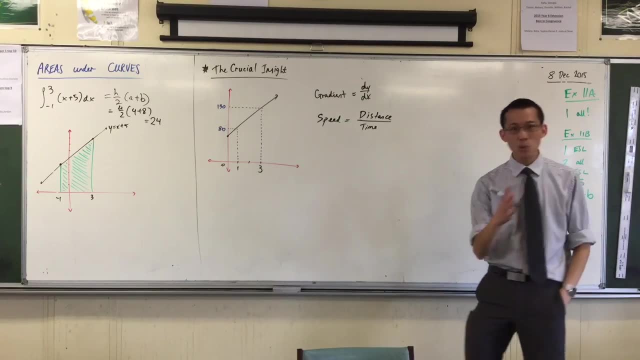 right. he starts at this object starts some distance away from the origin- right, wherever, that is okay. You designate some origin. After one hour it's 80 kilometers or 80 meters or whatever unit you like: 80 away from the origin. 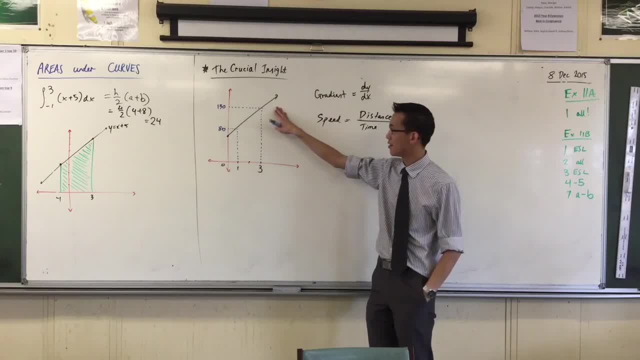 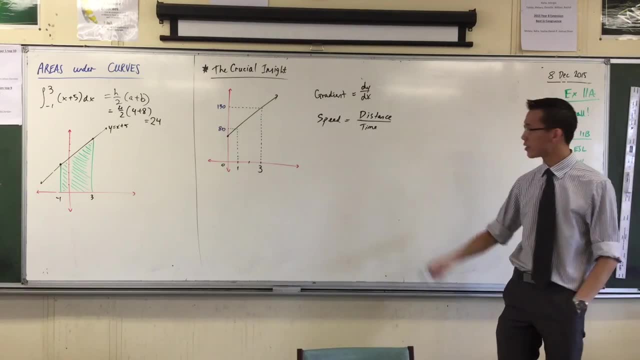 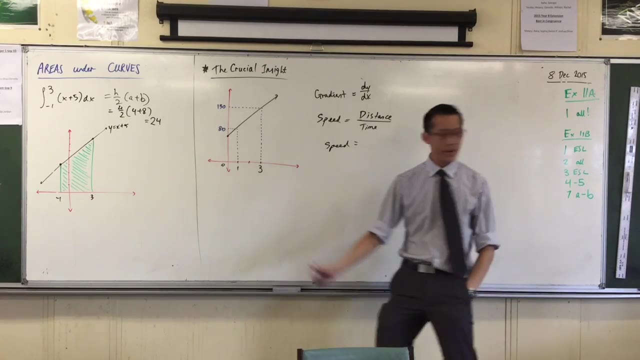 and after three hours it's 130 units kilometers. Actually, we'll just go with kilometers and hours away from the origin. okay, Now how would I work out the speed of this object? I would say that the speed is well between the first hour and the third hour. how far has it traveled? 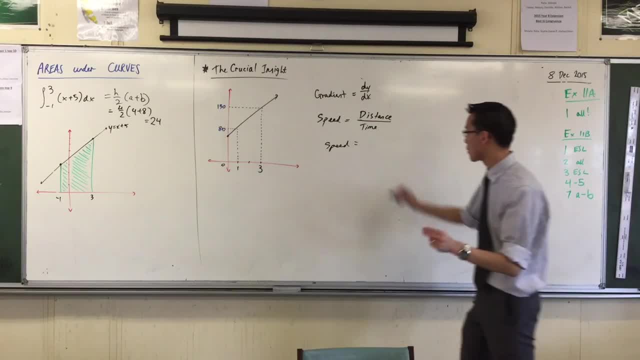 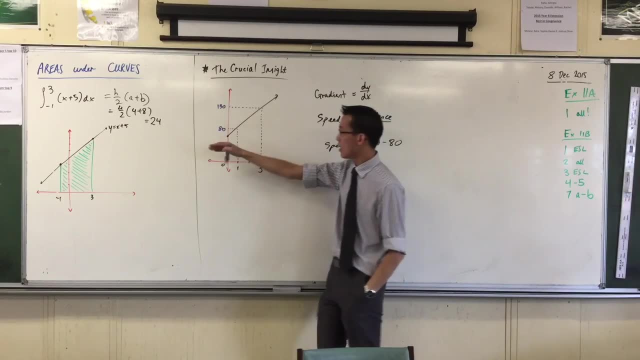 Fifty, Fifty, Very importantly, I'm going to write down that the 50 doesn't just come from 50, it comes from 130. take away 80. It comes from that difference. there, right Where I started, where I ended. 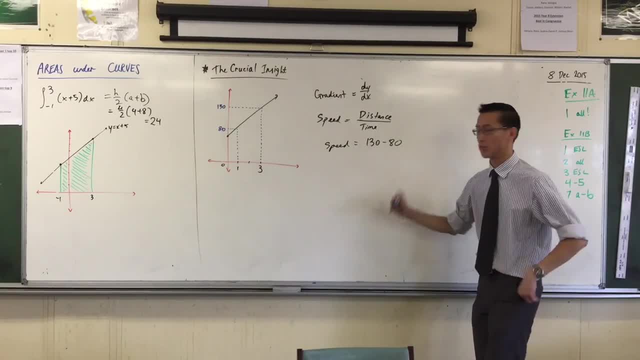 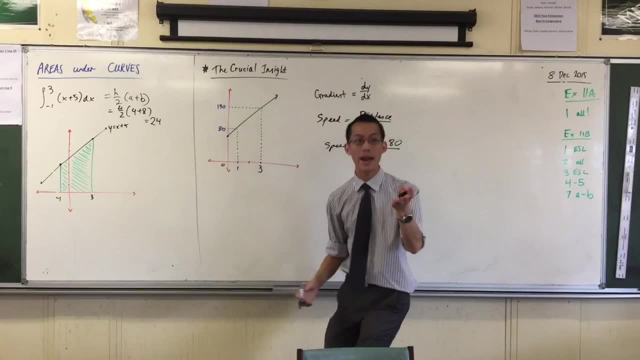 I compare those two, I take the difference and that's what gives me the total distance. I'm going to divide that by what was the total amount of time that I was traveling. Two kilometers to cover that, And the answer is two. and where does the two come from? 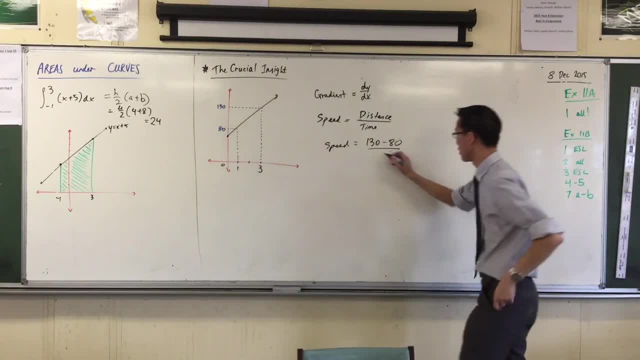 Answer: three take away one. So it's this quantity here. Three take away one, That gives you 50 over two, which is 25.. And I suppose I could call that kilometers per hour. okay, That's the speed that I'm interested in. 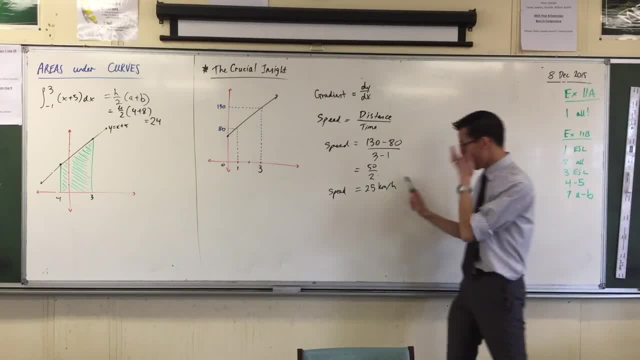 Now I want to take this idea of speed right. If I've got speed here, because this is a constant travel graph, it's traveling at constant speed. I want to draw, rather than a graph, that has distance against time. I could compare speed to time, okay. 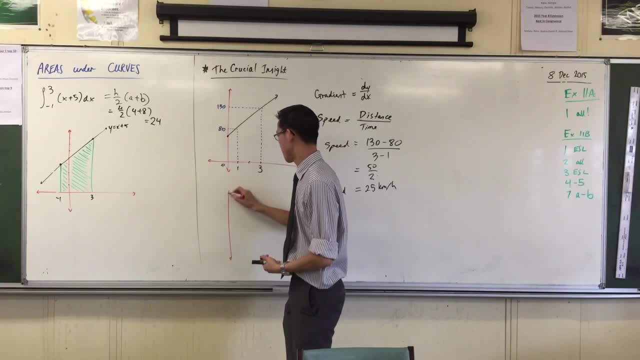 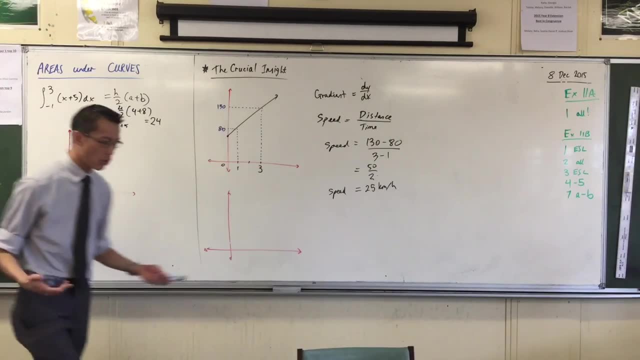 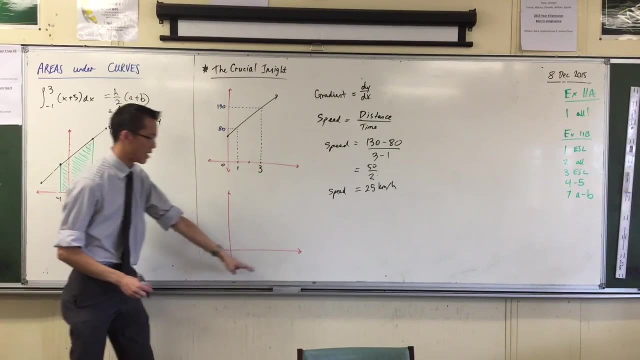 So just really quickly underneath here, it's a yes, okay, I can draw, rather than a time distance graph, right, I can draw a time speed graph. okay, Now, the speed is always 25 kilometers per hour, so it happens to be a very, very boring graph. 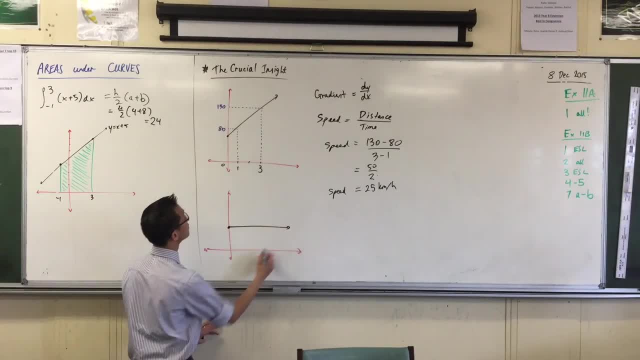 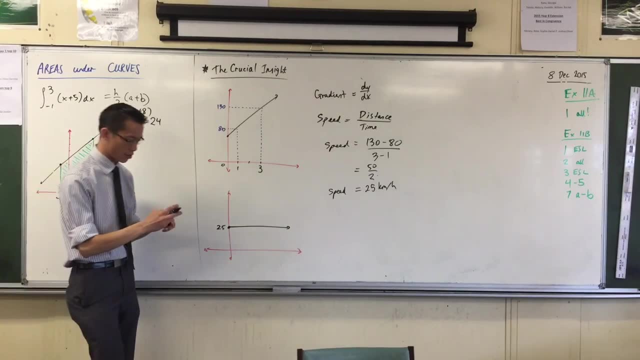 It looks like this: Yes, interesting, right, Okay. now here's the important thing I want to get across to you, Actually many important things. one of many, This is time distance and this is time speed. Now you remember what I was trying to say. 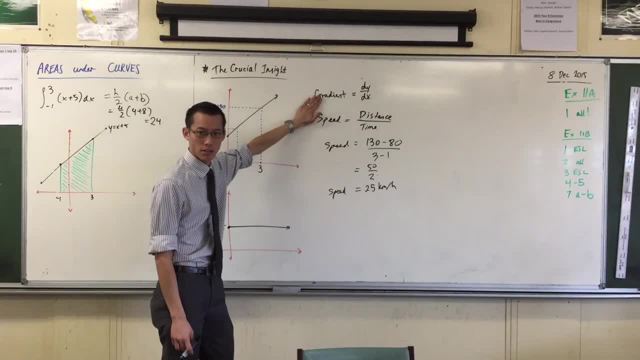 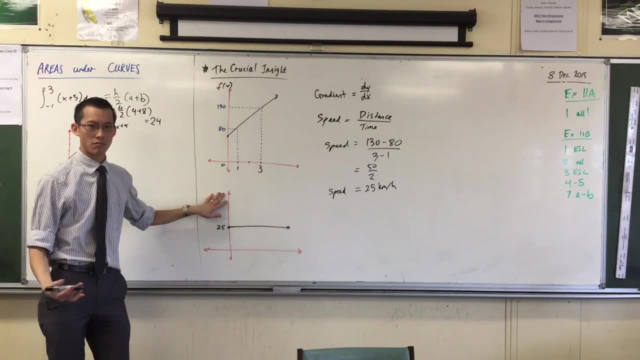 Speed is just about how you're changing, which is exactly what gradient is telling you, right? So I could call this: for instance: if this is my original function, then this is the gradient function, right? So I would call that: f dash. 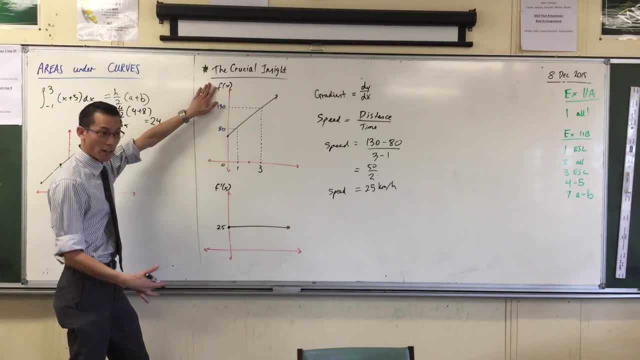 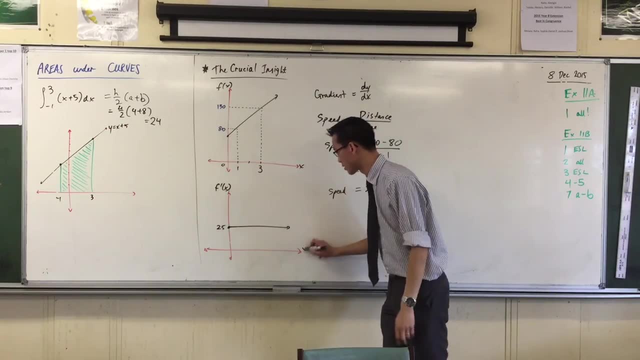 Are you okay with that? So, distance, the function, speed, the gradient function, right The derivative, And both of these are x's. okay, Now I've drawn them. that's why I've drawn them vertically, opposed to each other. 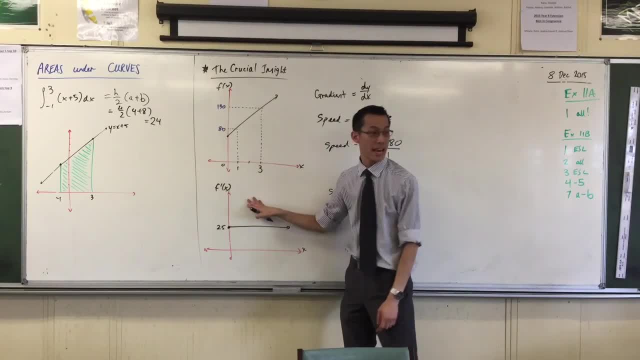 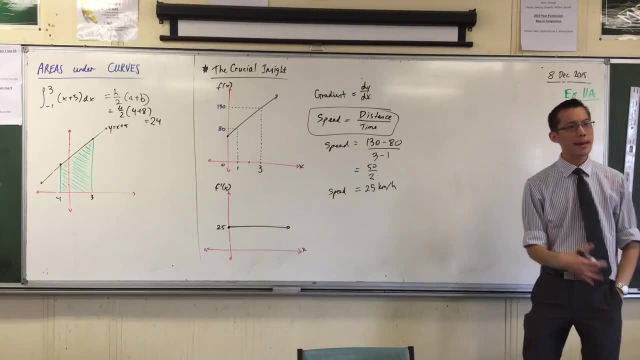 just the same way that you have drawn f and then compared it to f dash. Okay, no big deal. Now here's where we're going to push on this and squeeze some insight out of it. If speed equals distance over time, then it doesn't take that much imagination. 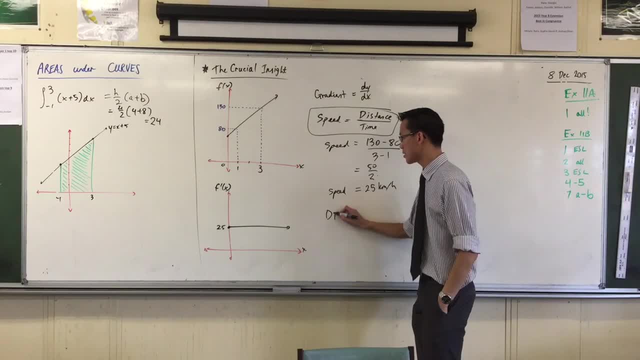 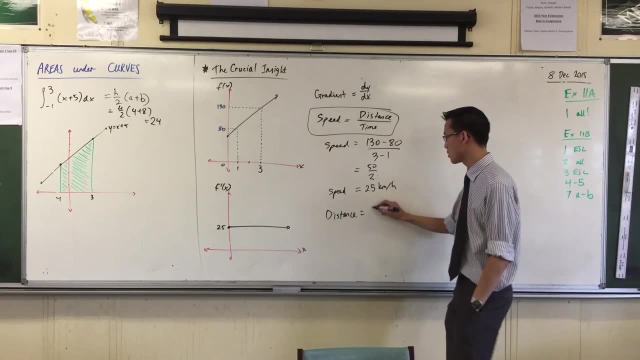 to try and solve this in reverse order and say: what's distance equal to in terms of the other two Speed times time. Yeah, you just multiply time across, right? So I would say: speed times time. Okay, does that make sense? 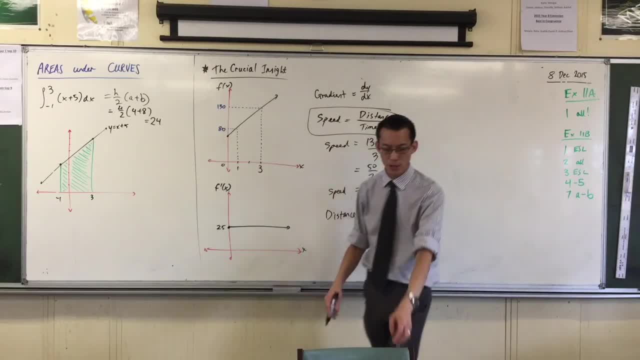 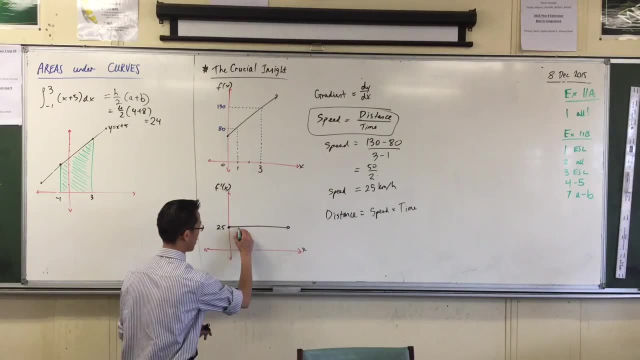 So, for instance, if I were to solve this particular question, but solve it in reverse, right, I could say: well, let's come down to this graph here, and for one it's going to go to about there, right, And three is going to go to about there, okay. 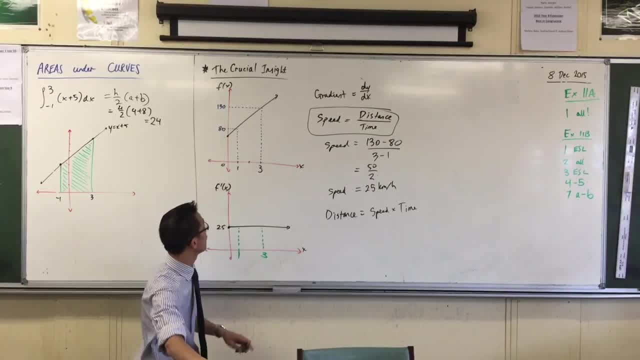 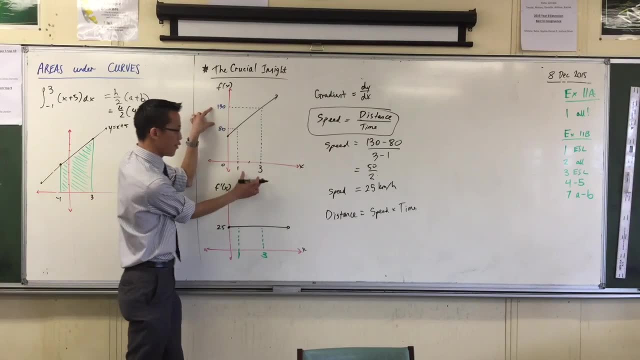 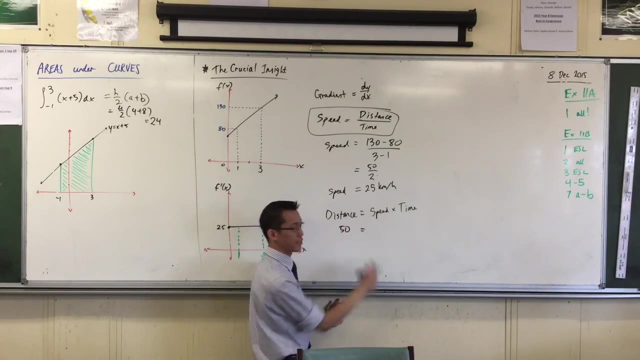 So this here: what am I solving For this particular set of numbers here? I had a distance of 50, that distance there over a time of two hours. Do you agree with that? So what I had was distance was 50, right. 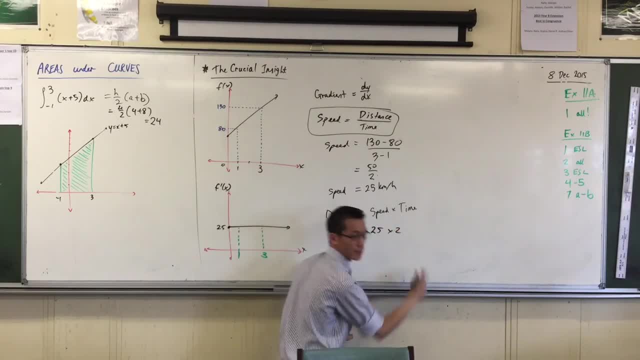 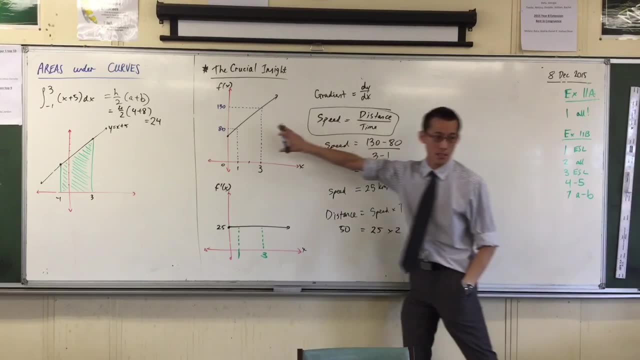 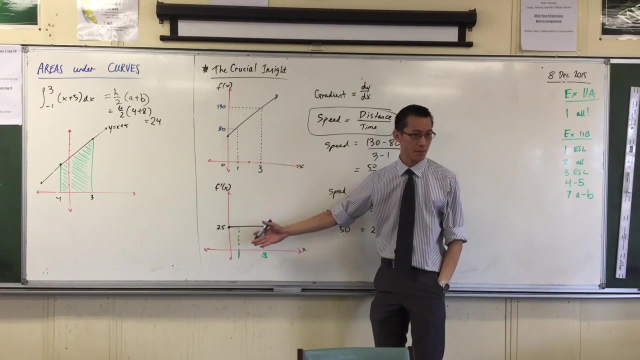 Speed was 25.. And I was travelling for two hours. okay, Now here's the crucial insight. okay, We know what this means on this graph, It's about gradient. What does this mean on this graph? The answer is this statement here: 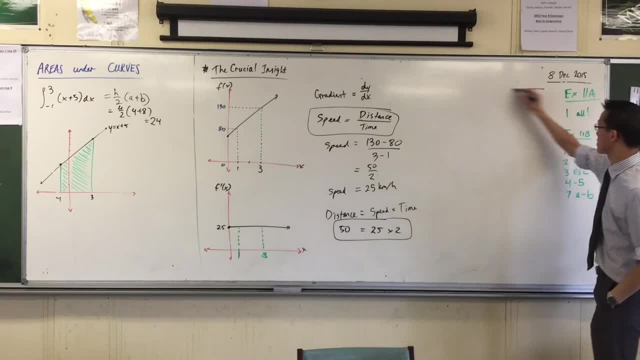 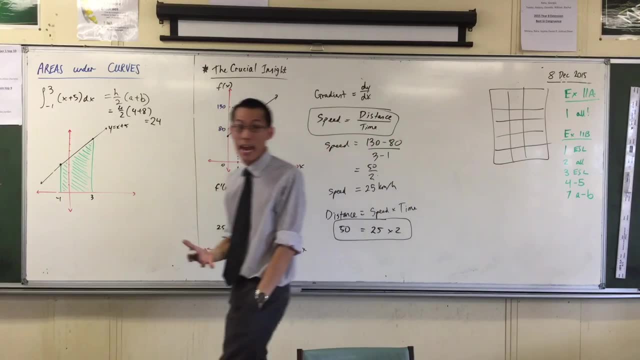 should look familiar, shouldn't it? Right back to the beginning of this lesson, I drew this thing right And I said that multiplication is really about well. it's used to understand area right. Area 50 equals 25 times 2.. 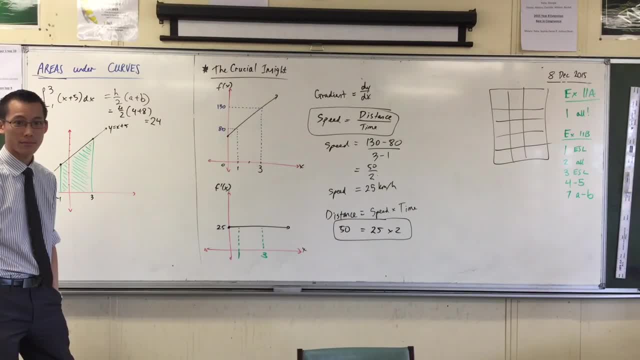 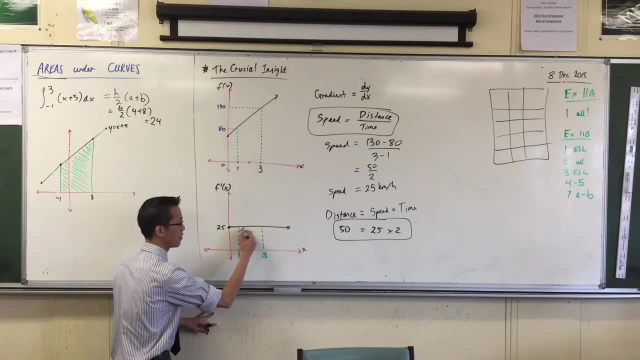 This is an area, isn't it? What area is it? It's the area of this guy in here. It's the area under this particular curve. Do you see that? This area under the curve is what this tells me? okay? 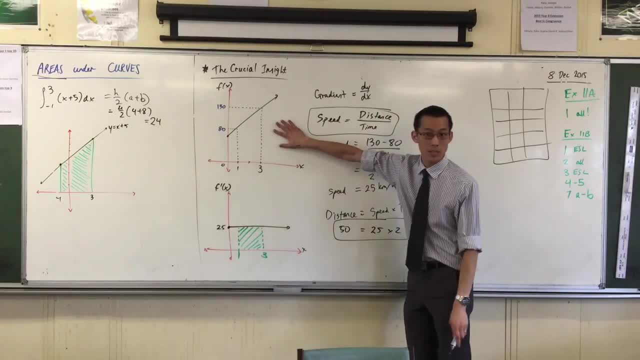 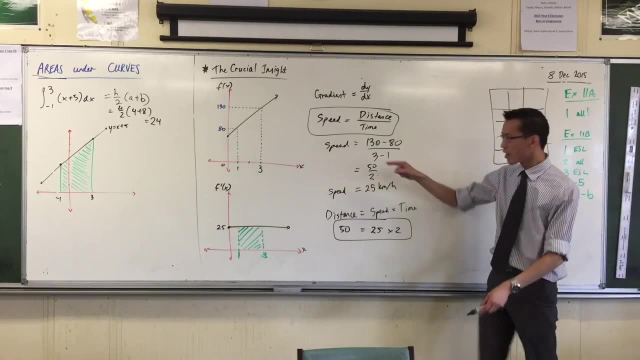 Now, I knew all of the numbers here, I knew exactly what was happening here and therefore I could draw some conclusions off of this right. But what this is suggesting is that, like, how did I go from here to here? Answer: I differentiated. 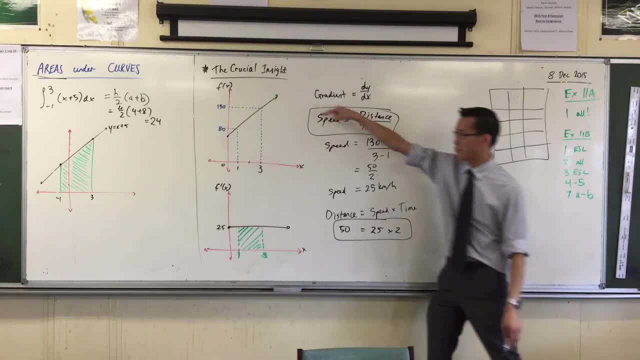 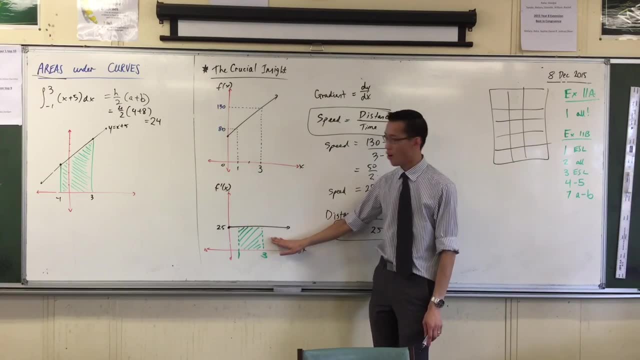 That's how. that's what speed is right. I differentiated going down here In order to work out the area from this right. all I need to know from here is now: stop, stop, stop. What is on this in this? I've got three numbers here. 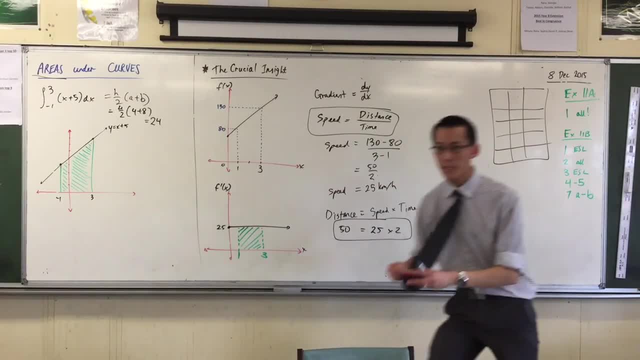 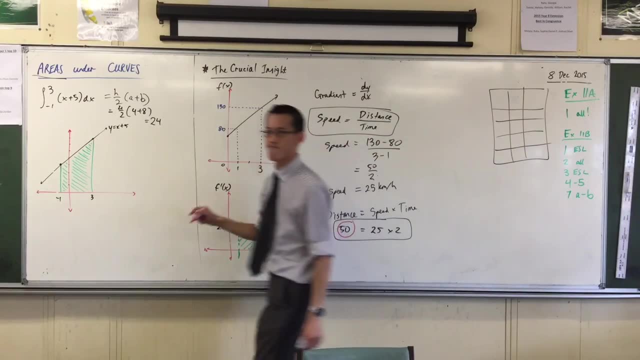 Which one's the actual area: 50.. It's 50,, right? That is the actual area. Where does 50 appear on this graph? Answer: yeah, and this is why I highlighted this. right, It's the total distance covered, right. 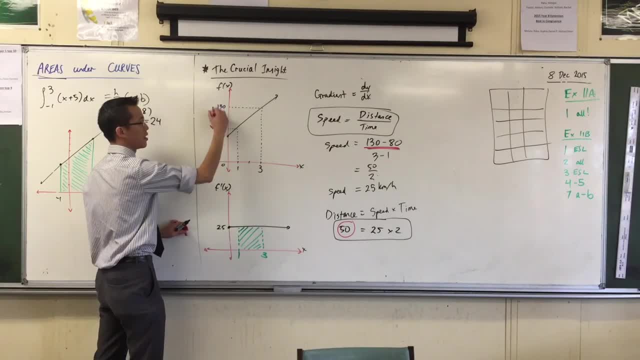 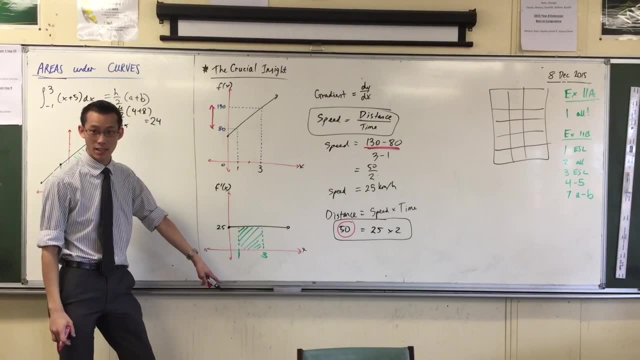 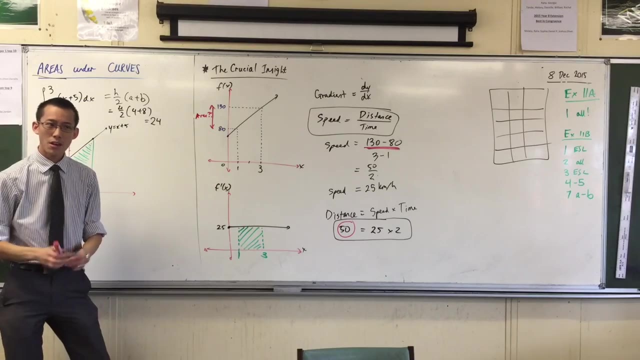 It's the start point and the end point compared, right, That distance there, this is the area down here. Okay, so what's going on here? right, I've chosen a simple example, I've chosen a straight line, okay. 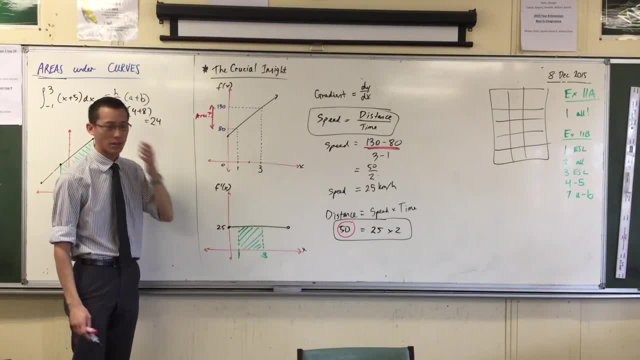 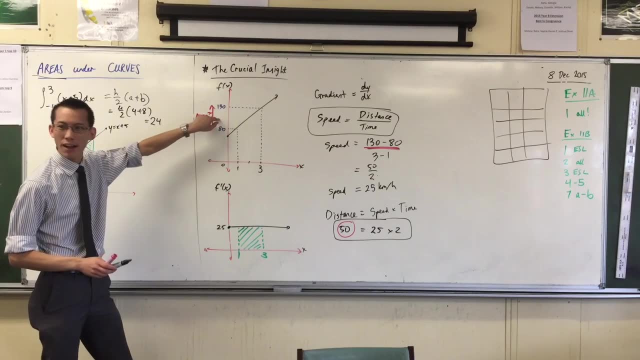 It wasn't even inclined off like that. That's why I just got a simple rectangle. okay. But if I want to work out the area under the curve, all I need to work out is having gone backwards from differentiating, which we gave this a name. 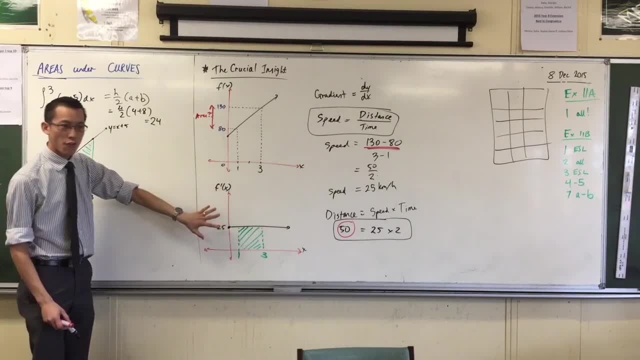 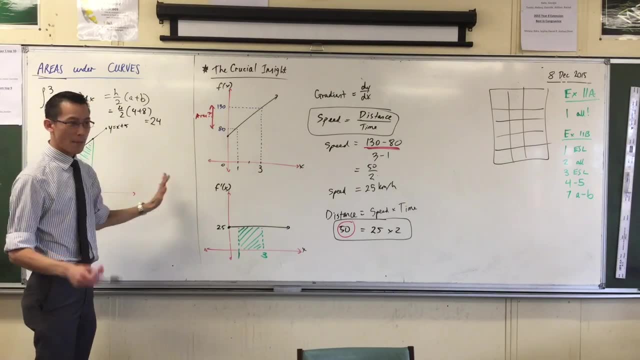 we called it anti-differentiating. right From here to here, all I need to know is a start and end point. A start and an end point. okay, Now remembering that to go from F to F dash is differentiating right. 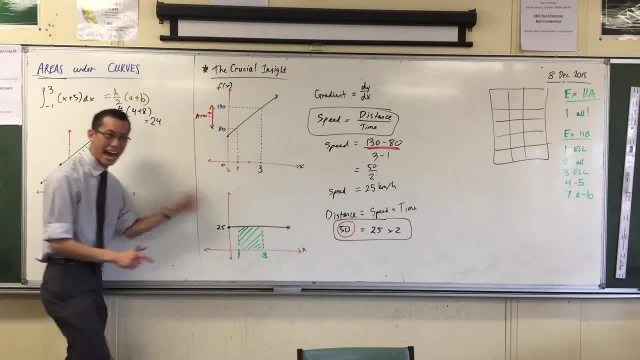 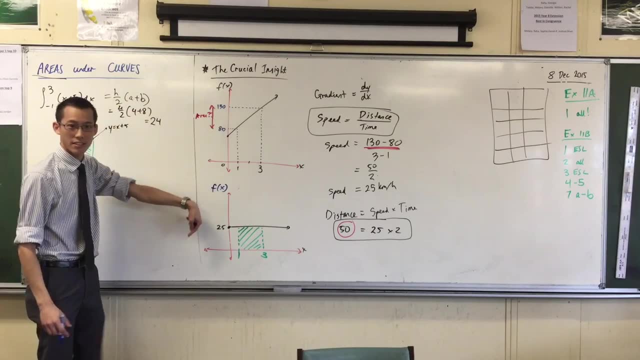 I can just rename these things right. If I call this the actual function I'm interested in, let's call this F right. Then the function I came from that differentiates down to this guy is the primitive. I call him capital F right. 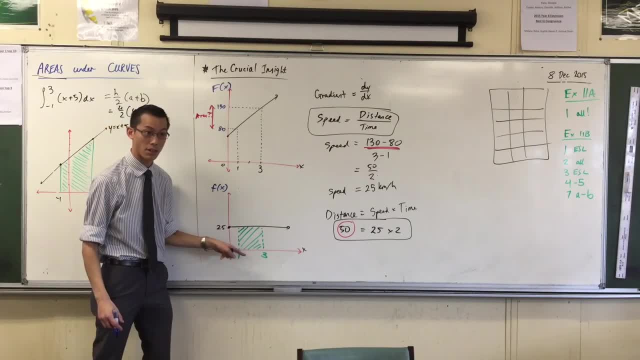 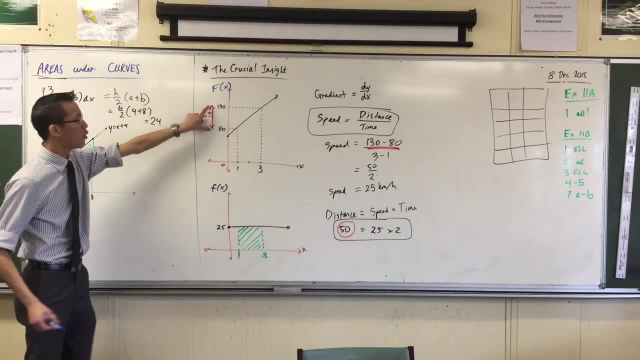 So if I start with this and I want to know this area under the curve, if I can know about the thing that was anti-differentiated, to get to climb up the ladder, all I need is these two values. Okay, So therefore, 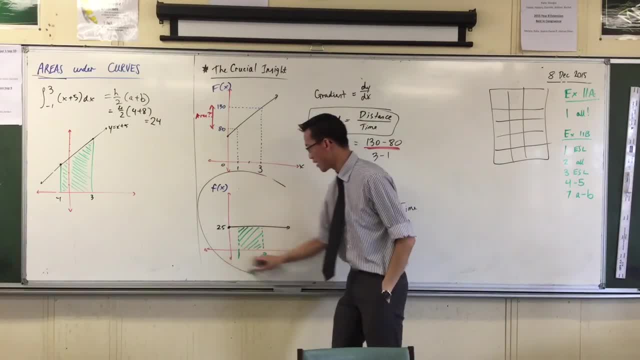 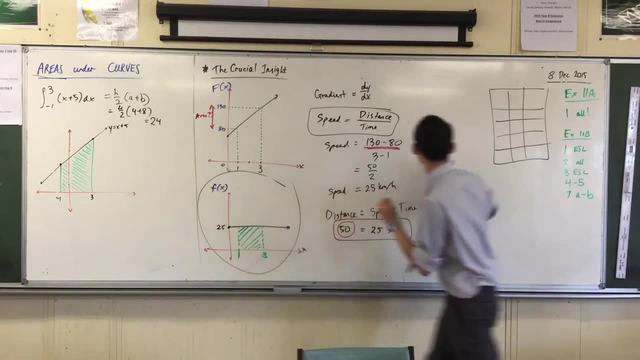 how would I state? by the way, how would I state this area under the curve, Like I know numerically what it is, but in integral language, which is all about areas under curves, how would I state it? Number one: start the integral sign. 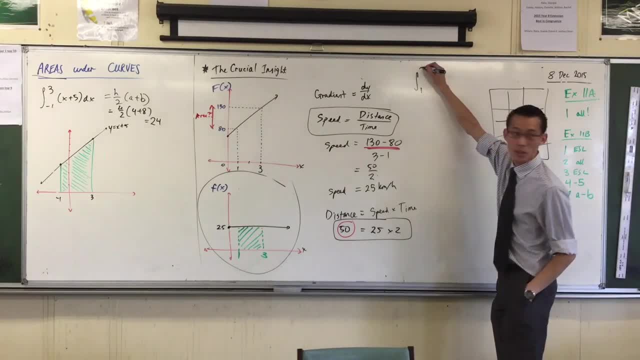 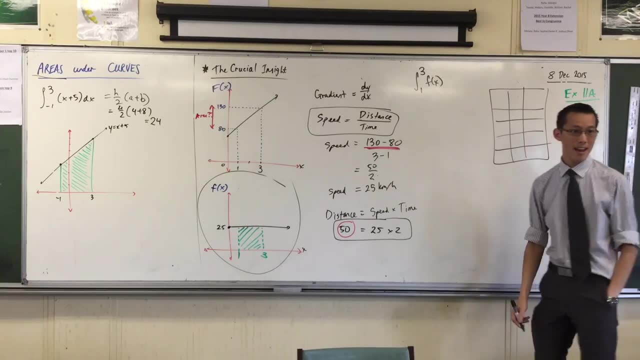 What are my boundaries? From one to three. Now, the thing I'm integrating is this guy right F of X, And I'm doing that with respect to X. There's those little widths Crosses, right Now, what is it actually equal to? 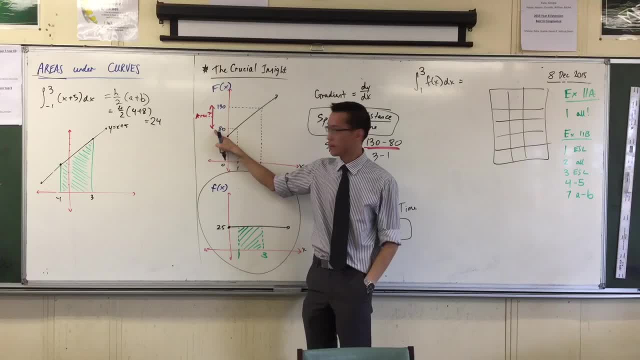 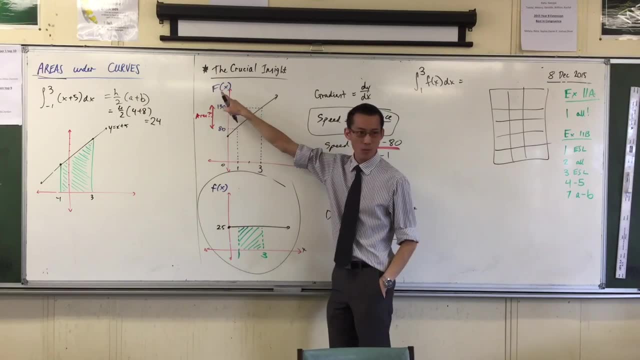 Right, Well, I needed the start point. I need the end point Really. it's end, take away start. Does that make sense? Okay, Now, where did I get 80 and 1 and 30 from? They came from these values.